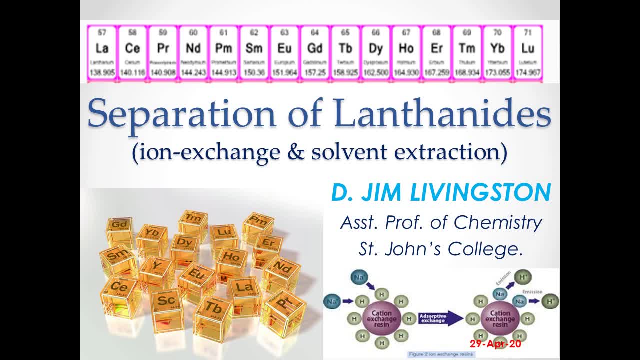 Hello, dear students, again, I welcome to this online class. We are going to see about the separation of lanthanide ions using ion exchange method and solvent extraction method. In our last video we have discussed about the basics of ion exchange chromatography in the separation. 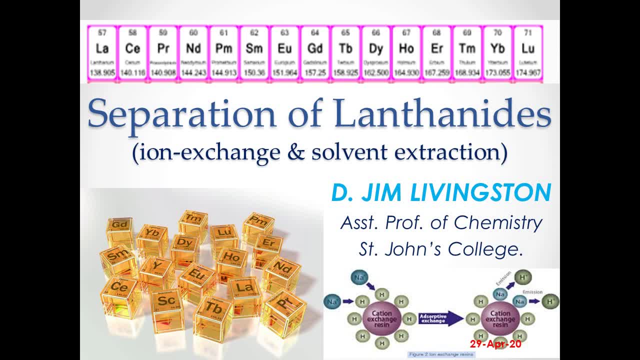 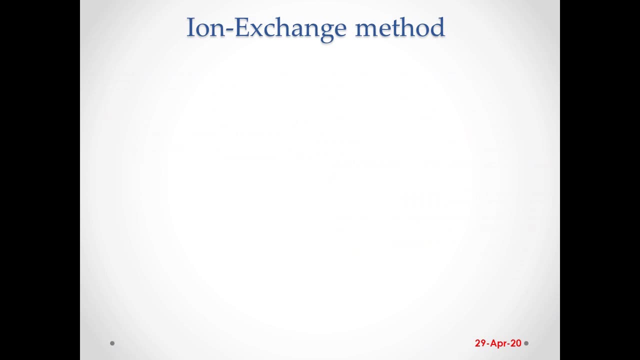 of compounds. Today we are going to learn how this ion exchange method is used in the separation of lanthanide ions. In this slide I want to refresh you about the ion exchange method we have learnt in the previous class. This apparatus is called as the glass column, Here the glass 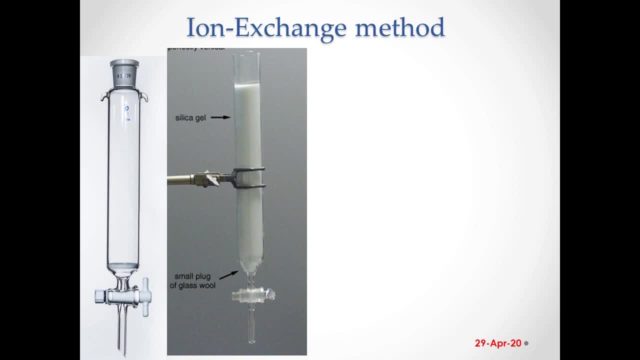 column is filled with the stationary phase. Here silica gel is used as the stationary phase. This is the glass column. Here the glass column is filled with the stationary phase. This picture represents the mobile phase is added into the stationary phase. So after. 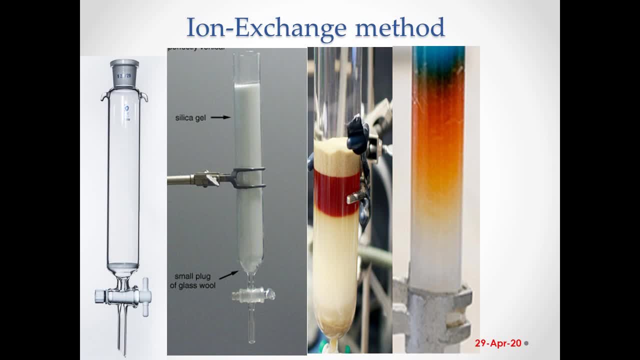 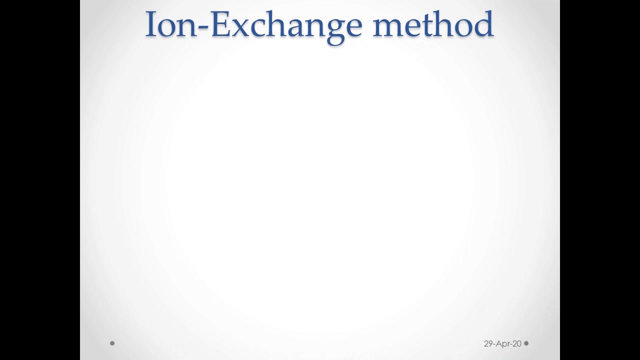 some time. the different chemical components present in the mobile phase is being separated. As you can see, different color bands are arises. Finally, the column is eluted with another solvent so that the different chemical component can be removed. Now we move on to the separating of lanthanide ions using ion exchange method. In this picture, 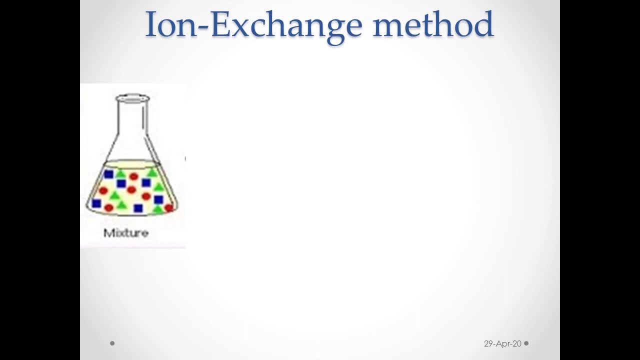 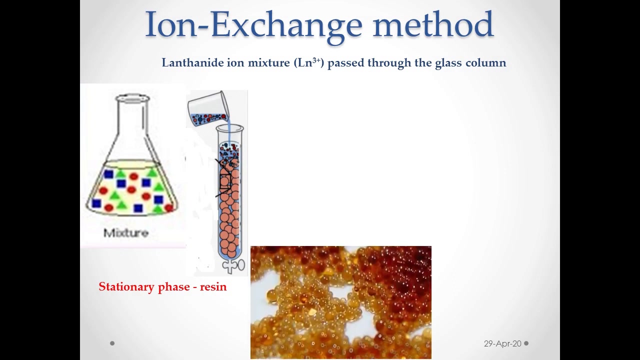 the mixture of lanthanide ions is taken in a beaker and this lanthanide ion mixture is passed through the glass column. Here the stationary phase is a polymer resin and it is represented as brown color circles. Here it is the polymer resin, Now using this glass column. 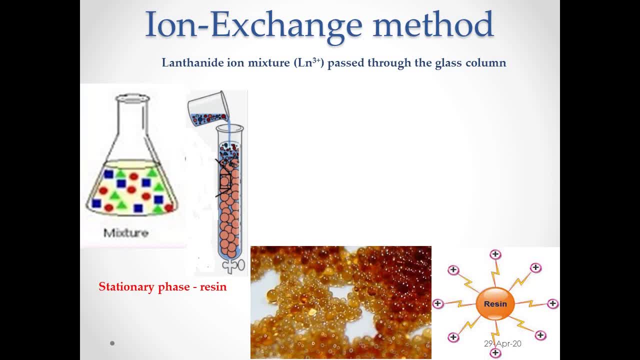 and the resin you see it is. it contains a positive charge group functional group present in it. that means cation. the lanthanid ions are dissolved in water but our stationary phase, that is, the polymer resin, is in a solid state after the lanthanid ions is passed through or poured into the column interactions. 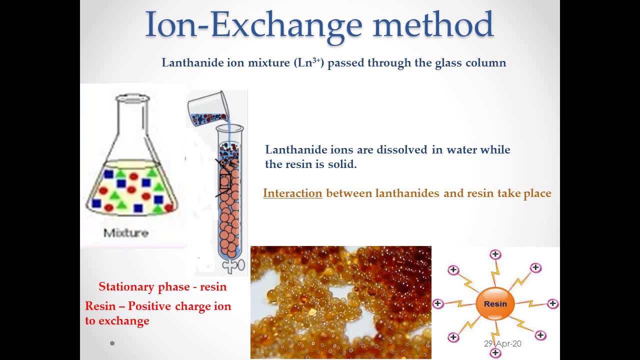 are taking place between the lanthanide ions and the resin. that means there is an exchange of lanthanid ions with the positive charge ion present in the resin. this is the equation that represents the exchange reaction. rh represents the positive charge ion present in the resin. 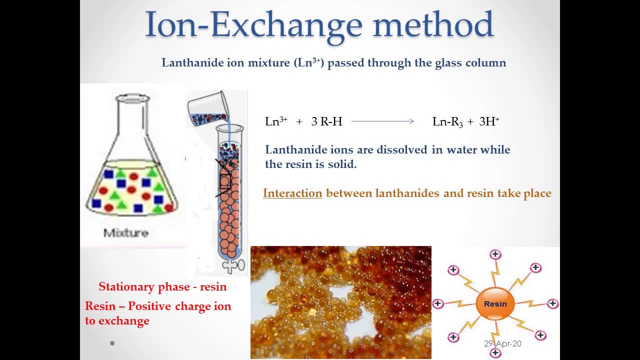 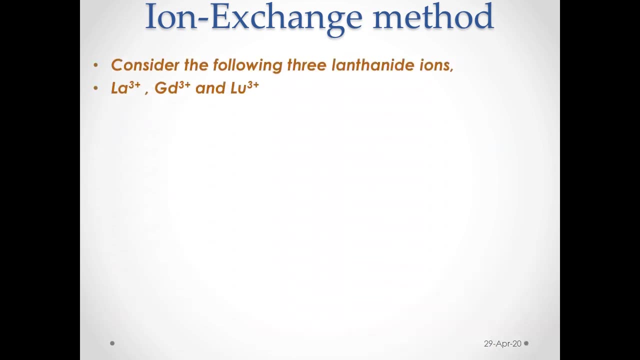 h plus is the positive charge ion present in the resin. so after the exchange reaction, our lanthanum ions, or lanthanoid ions, is attached with the resin, while the h plus ions is removed. for our example, let us consider the following three lanthanid ions: lanthanum gadolinium and 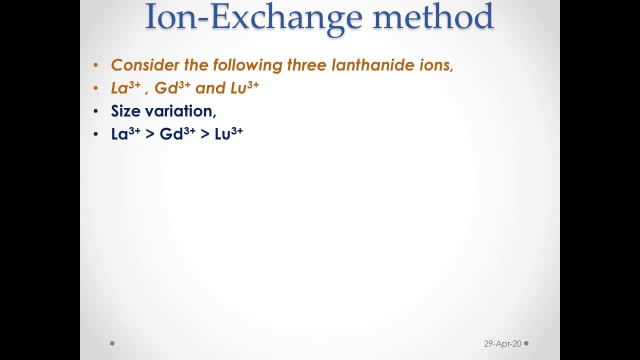 lutetium 3 plus ions. as we know, from lanthanum to lutetium, the size decreases. therefore, lanthanum 3 plus is larger in size, while a lutetium 3 plus is smaller in size. and now we are dissolving all. 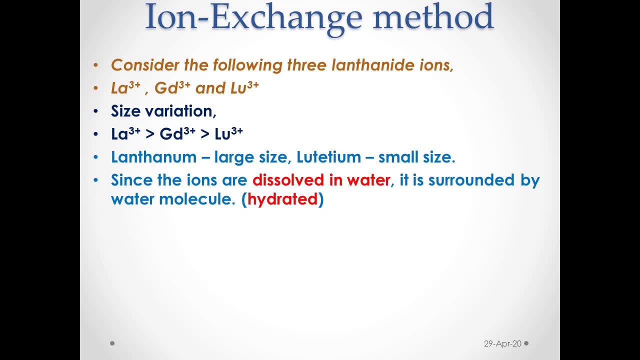 the lanthanoid ions in water. therefore, all the lanthanid lanthanoid ions are surrounded by water molecules. in other words, all the lanthanoid ions are hydrated. it is well known that smaller the ion, greater will be the hydration. as we can see in this picture, lutetium 3 plus ion is the smallest ion in the lanthanide series. 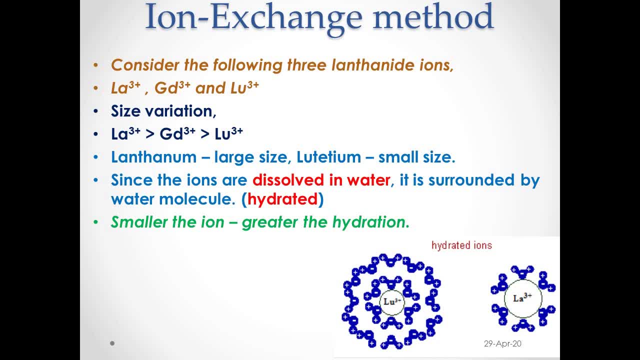 and it is surrounded by a large number of water molecules. hence the hydrated lutetium 3 plus ion is bigger in size, but lanthanum 3 plus ion, the largest ion in the lanthanide series, is surrounded only by a smaller number of water molecules and it is the ion having smaller 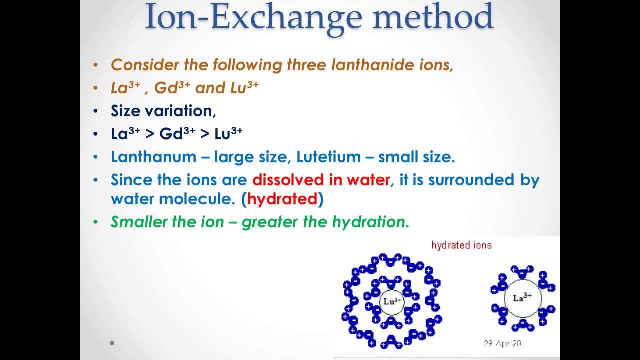 and it is the smallest or smallest hydrated ion. now, another one important concept is: the smallest hydrated ion is strongly binded to the resin, with the resin. therefore, in our case, lanthanum 3 plus ion, which is the smallest hydrated ion, is attached strongly with the resin and therefore it is held at the top of the column. 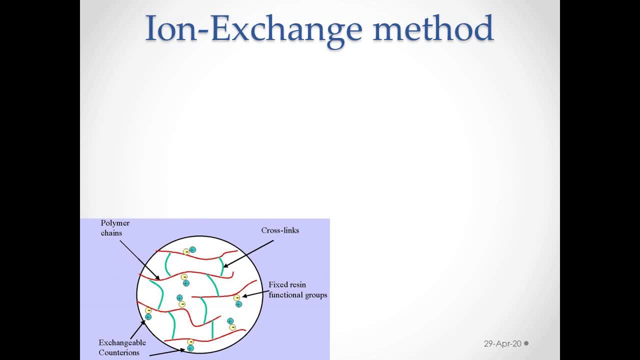 this picture shows a single molecule of the polymer resin. the red color line shows the polymer chain which has, which is cross-linked, and the positive charge shows the exchangeable counter between the two molecules. that means the h plus in our case, and this is the picture in which the 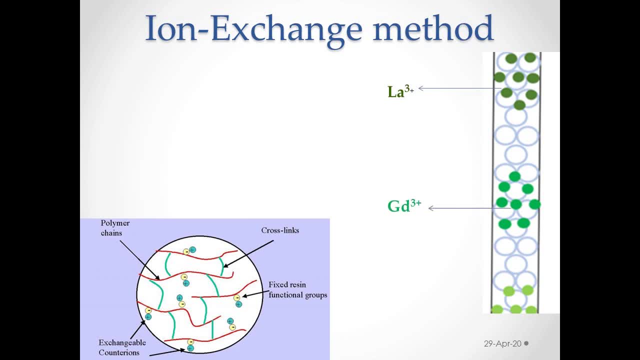 lanthanum 3 plus ion is held at the top layer, gadolinium is held in the middle portion, while lutetium 3 plus ions comes to the bottom, because the interaction between the polymer resin and lutetium is very weak. so when we elute this column with a suitable element, 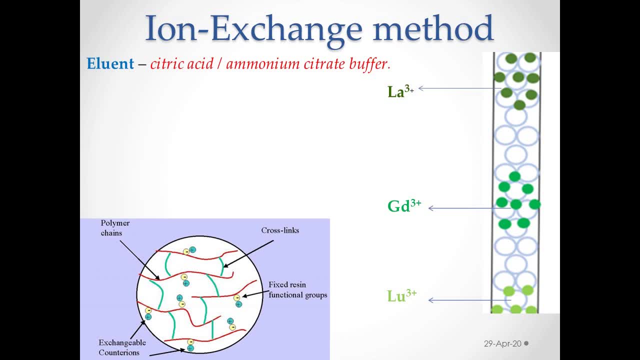 in our case, we use citric acid and ammonium citrate. buffer lutetium, which is held at the bottom, comes out first, and this is equation shows the interaction between the element and our lanthanate ions attached in the polymer resin: r represent the resin and la represent our lanthanate. 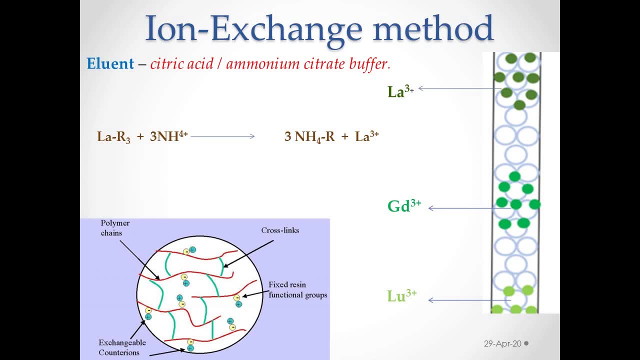 ions and after the element is passed, our lanthanum ion is separated. so lutetium comes out first because it is held in the bottom, held at the bottom, while lanthanum, which has very strong attraction with the stationary phase, comes out last. so in this way we can separate the mixture of lanthanate ions into individual ions. 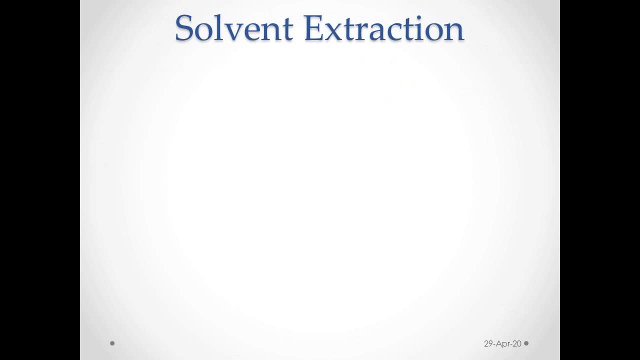 now we move on to the separation of lanthanate ions using solvent extraction method. extraction means the transference of a compound from either a solid or a liquid phase into different phase. here in this picture, you see a tea cup with the tea bag inserted into it. you know how this tea is prepared. 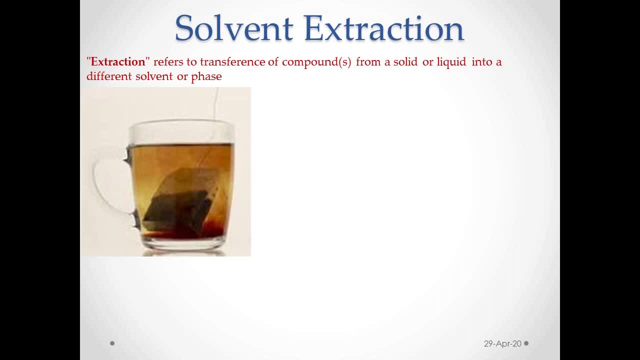 you have taken hot water in the cup and once you added the tea bag into it, the flavor and the color of the tea is transferred from the tea bag into the hot water. this is called as extraction. there are different types of extraction, as you see here: a liquid liquid extraction, solid phase extraction, acid based extraction, etc. we are interested in. 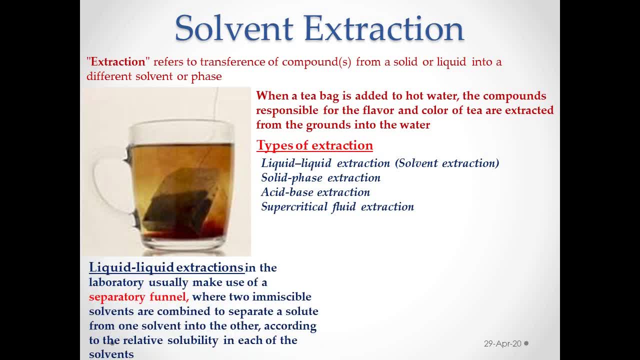 a liquid- liquid extraction. it is also known as solid phase extraction, solvent extraction. For carryout solvent extraction, we need an apparatus known as separating funnel. This picture shows a typical separating funnel. We also need two solvents, and the two solvents must be immiscible with each other. Therefore, one solvent must be water and another solvent. 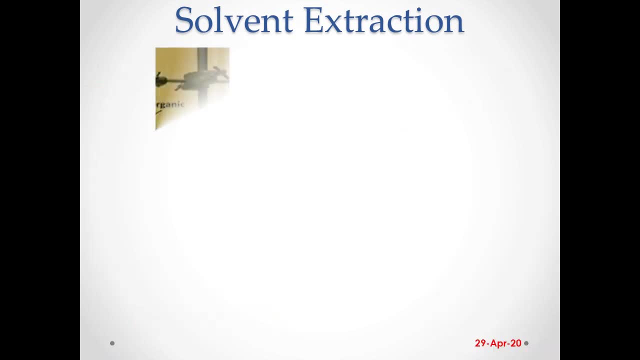 must be an organic solvent. Here, in this picture, you see a separating funnel with two immiscible liquid. The aqueous phase is held at the bottom, while the organic phase is held at the top, since the organic phase is less denser than water. Now I am going to explain the separation. 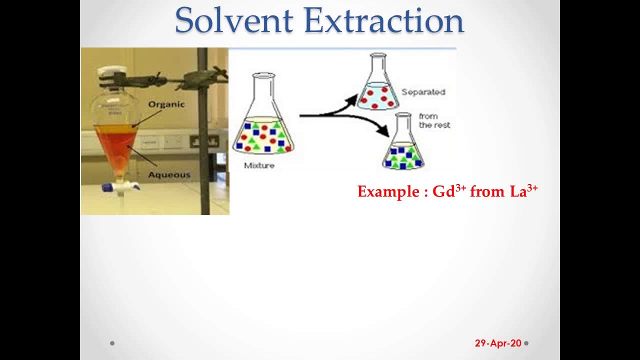 of lanthanid ion using solvent extraction method. Let us take how gadolinium 3+. This ion is separated from lanthanid ion. In this picture you see the separating funnel contains the aqueous phase. is represented in blue color shade which carries dark black. 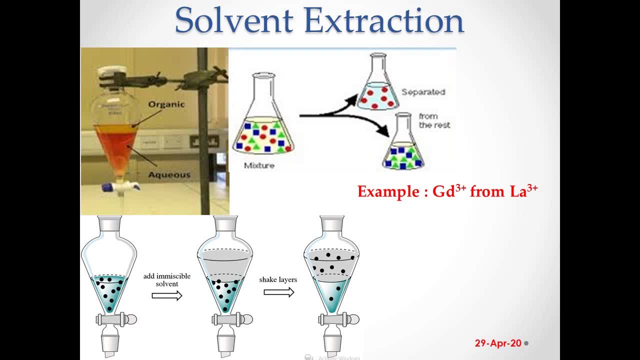 color circles representing the ions. After adding another solvent which is immiscible with water, usually an organic solvent, an ash color is used to represent the organic solvent. You shake both the solvents. After some time the dark black color solute particle from the aqueous phase is transferred into the organic phase. 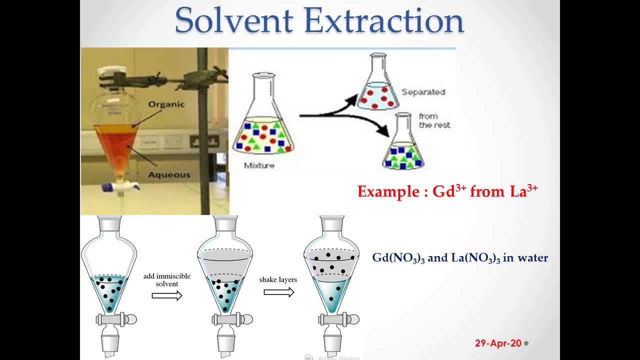 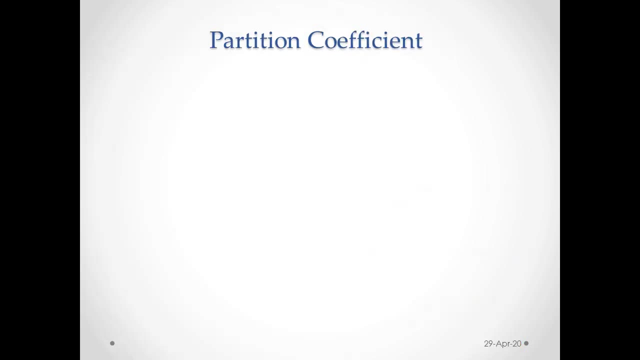 In our example, we take both the gadolinium and lanthanum nitrates dissolved in water, And our organic phase is tributyl phosphate salt dissolved in kerosene. Before moving into the further explanation of this solvent extraction, let me brief you. 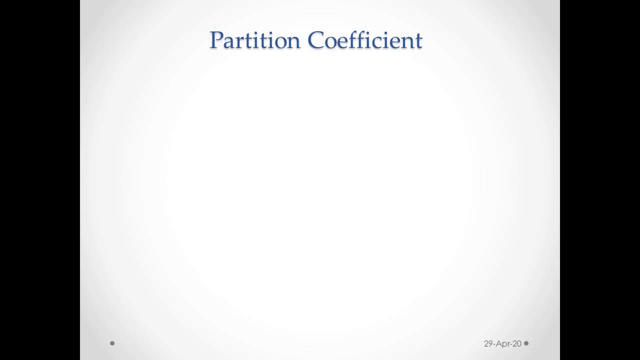 about another one important concept connected with this solvent extraction, which is known as partition coefficient. When a solution is placed in a separating funnel and shaken with an immiscible solvent, The solute particles dissolve in both organic layer and in aqueous layer. That means the 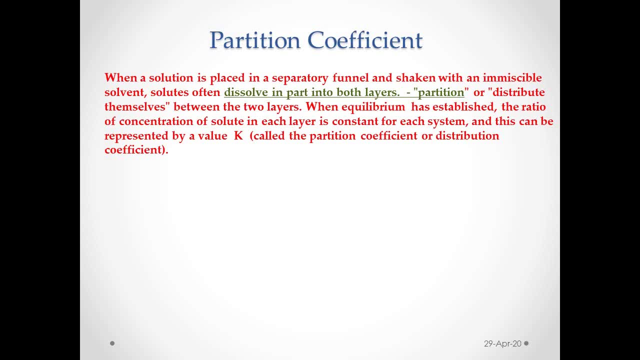 solute distribute between the two layers. So after some time an equilibrium is established. So, after the equilibrium has established, the concentration of the solute in both or in each layer is constant, And this is termed as partition coefficient And it is defined as the ratio. 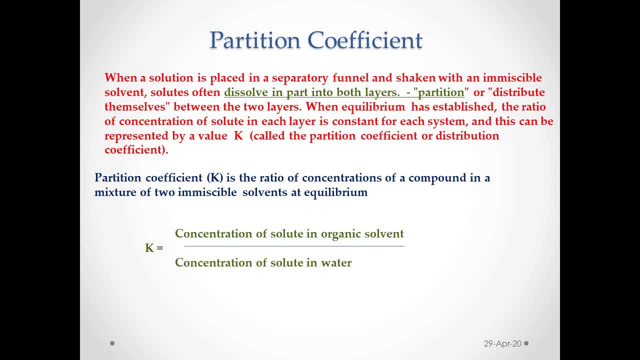 of concentration of the solute in organic solvent and the concentration of the solute in water. You see here, after some time some solute particles are dissolved in organic layer, while most of the solute particles are dissolved in organic layer. I must credit Professor Lisa Nicholas of Butte Community College, California, USA, for giving. 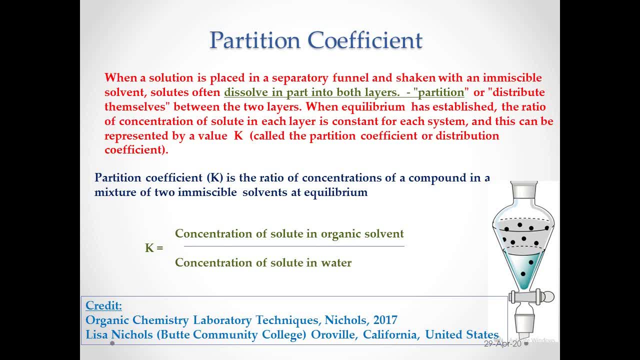 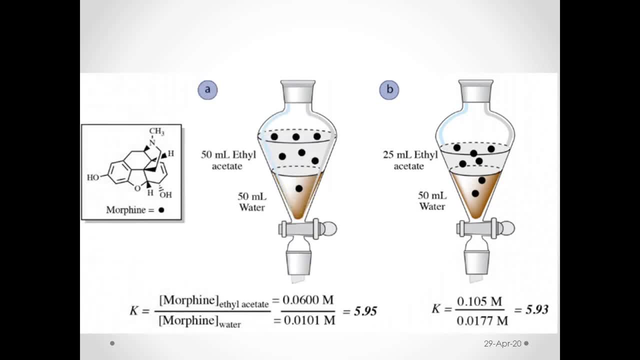 me permission to access some of the pictures And Theoretical parts from her book. Let me explain the concept of partition coefficient with a simple example Here. we take morphine, a chemical compound, and dissolve in water, And after adding our organic solvent, that 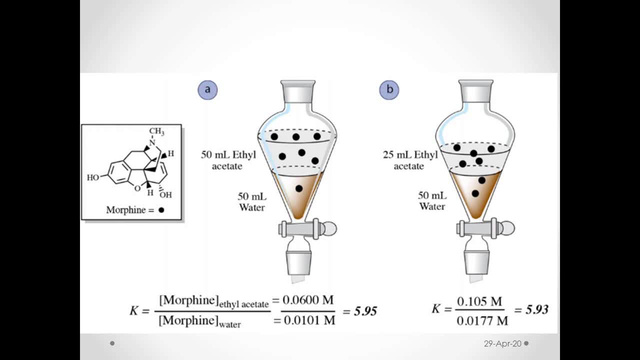 is ethyl acetate. shaken the two solvents after some time you see one molecule of morphine is present in 50 ml of water, while the rest are transferred into the ethyl acetate medium or ethyl acetate solvent. So there are six molecules of morphine and one in ethyl acetate solvent, while one molecule 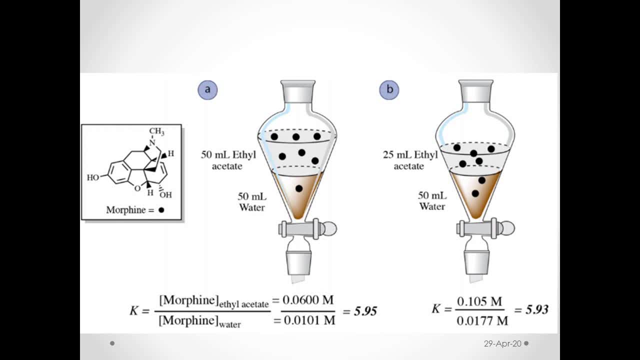 of morphine in Aqueous layer. Now we find the value of K. it is found to be 5.95.. And in the second part that is in In the Picture represented by B, This is the, The Volume of ethyl acetate is reduced to. 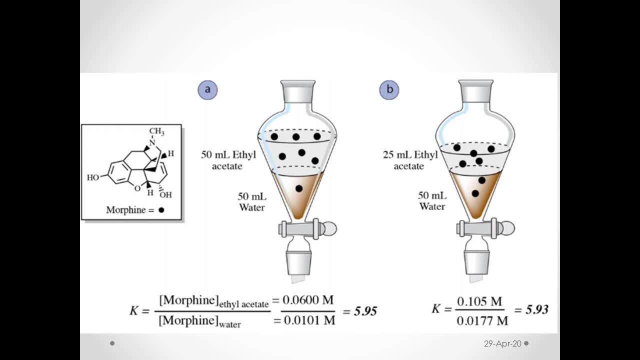 25 ml, While the volume of water is or remains same, That is, 50 ml. Now we find out the value of K. again, the value of K is found to be 5.9.. Which means The value of K, that is, the partition coefficient, is 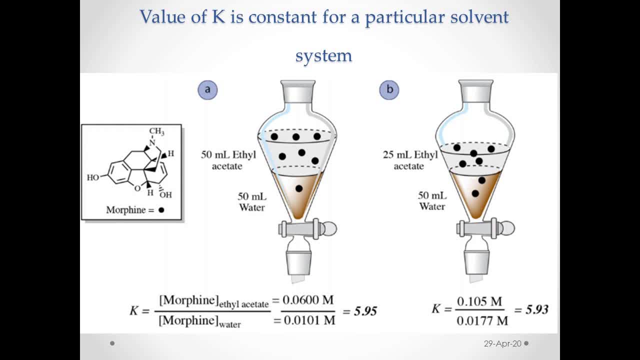 Constant for morphine Is constant Is constant, So for a particular solvent system. that means, in our case, if you take water and ethyl acetate as solvents, then how much volume of water or how much volume of ethyl acetate you take. 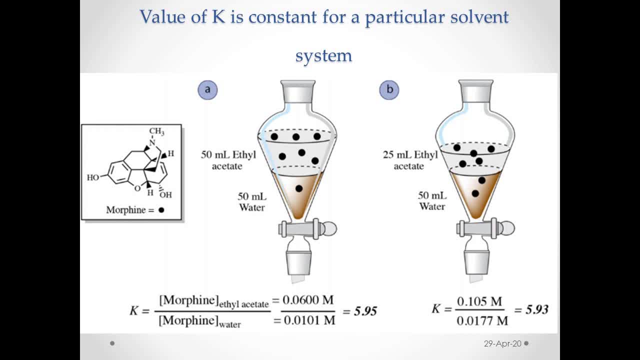 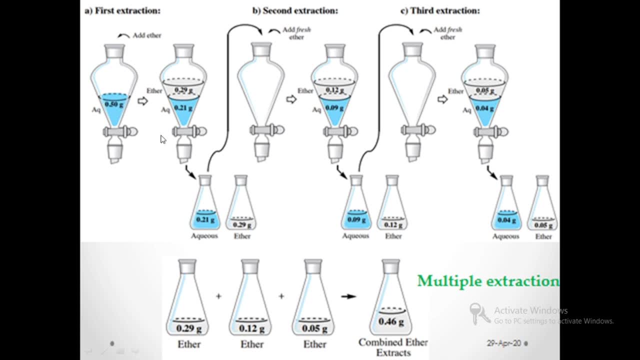 the partition coefficient for morphine in this system is 5.9.. In this slide you see you have a multiple extraction process. So in the first extraction process you have 0.50 gram of our solute dissolved in water and after adding the organic layer here we add ether- 0.29 gram. 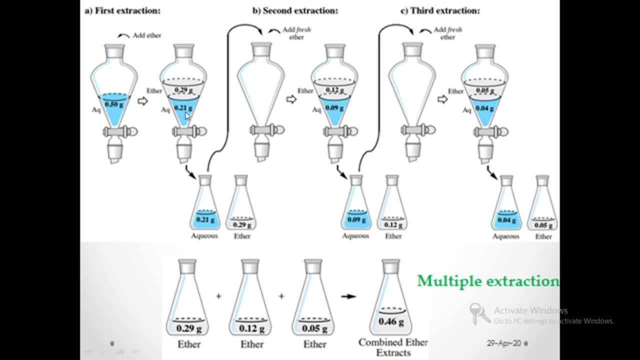 is transferred from the aqueous layer into the ether layer. Therefore, that means more than half of 0.29 the mixture is transferred into the ether layer. Now we separate the aqueous layer and ether layer into different beakers, Further proceeding into the second extraction process. this aqueous layer 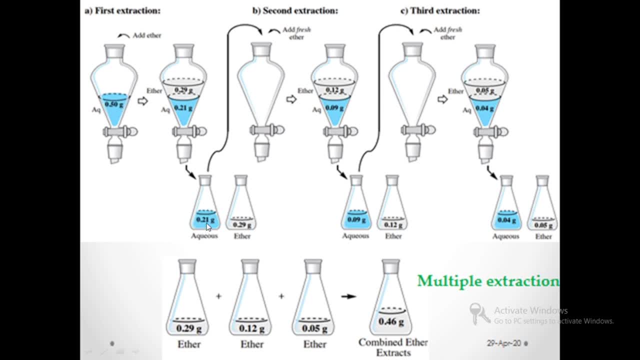